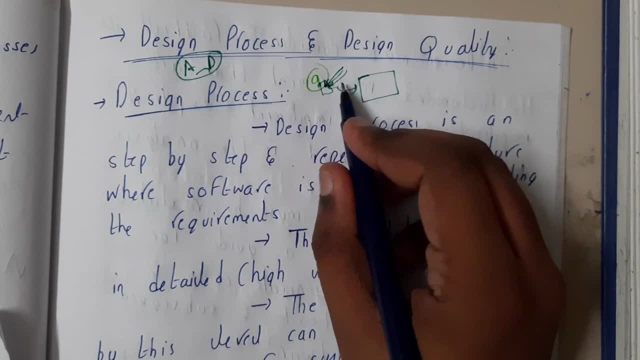 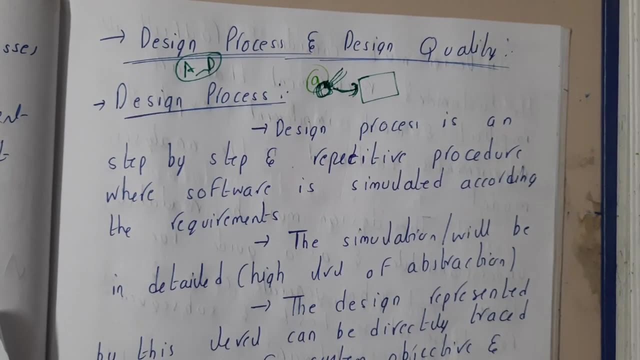 So the outer structure, the architecture, the model you will be designing in this step, guys. So, based on this step, only the architecture, design only and the user interface and everything the designs, only the coding is done. So, based on these designs, how you are designing them. 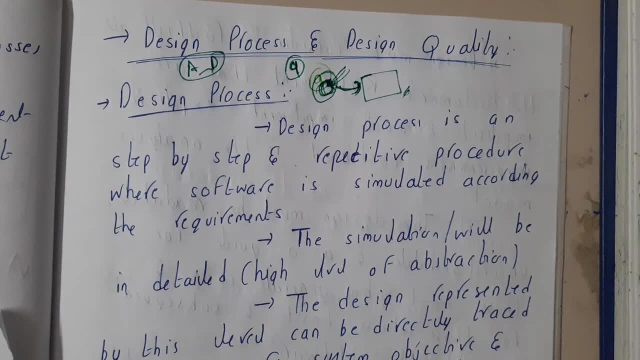 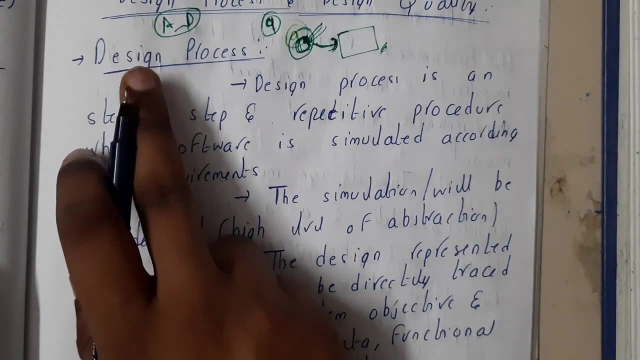 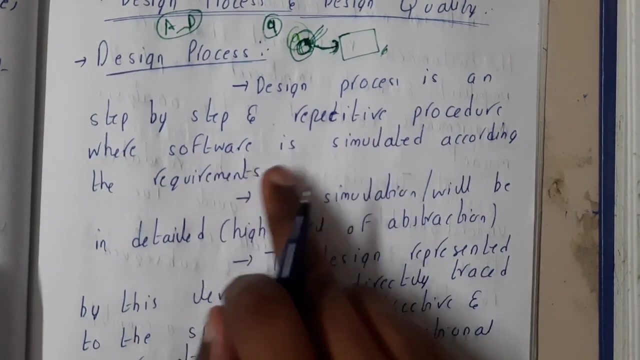 So, based on that, only So, basically, you will be getting your output, guys, okay, Okay, output is nothing but I am saying about, I am talking in terms of coding, Okay, so let us continue. So, design process: Design process is a step by step and repetitive process where the software is simulated according to the requirements. 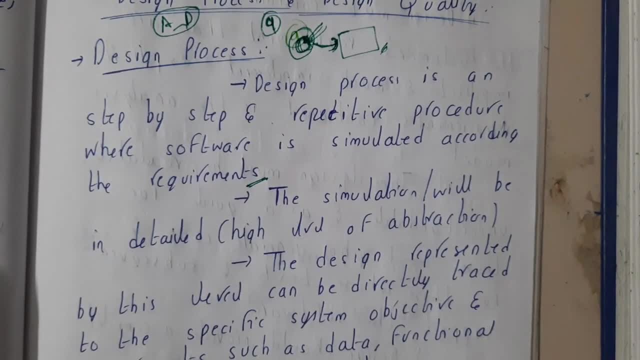 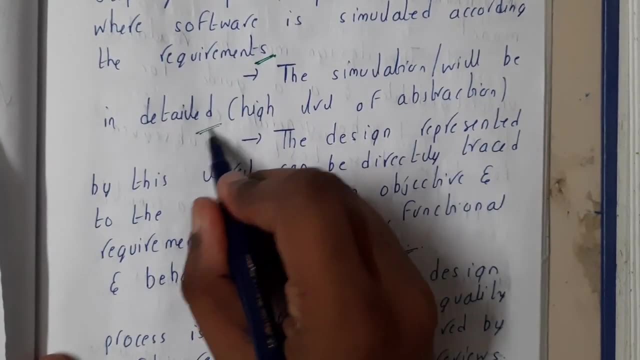 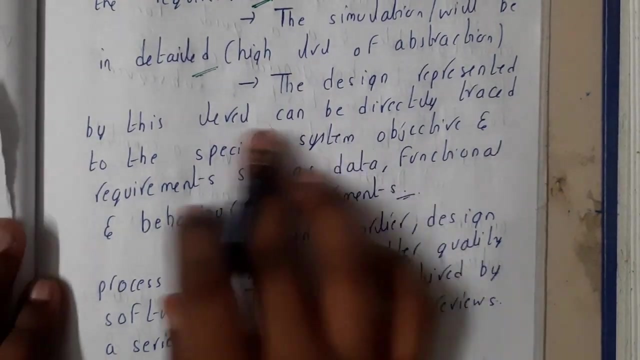 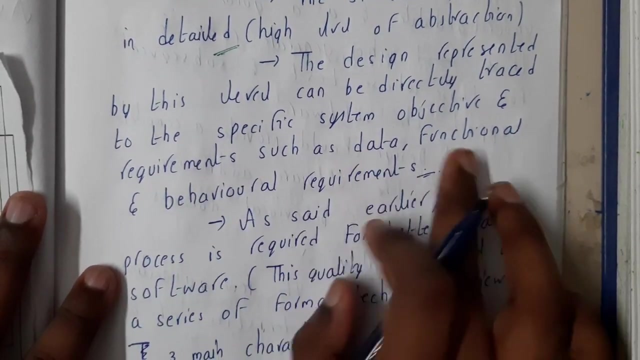 So basically you can say that here you will be making some kind of dummies guys. Okay, so the simulation will be in detail, high level of abstraction. So basically, Here you will be simulating in detail like the exact model. you will be making a duplicate guys. okay. so the design represented by the level can be directly tracked to the specific system objective and the requirements, such as a data function, behavior requirements, can be identified easily. 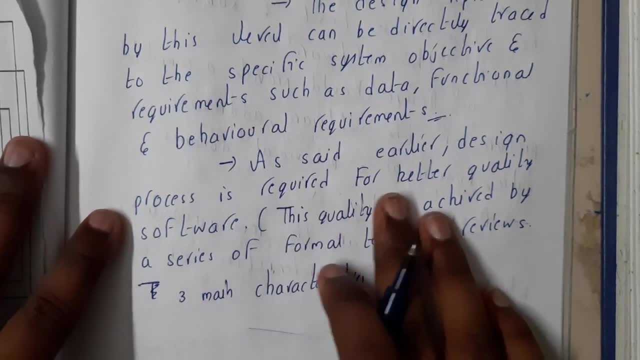 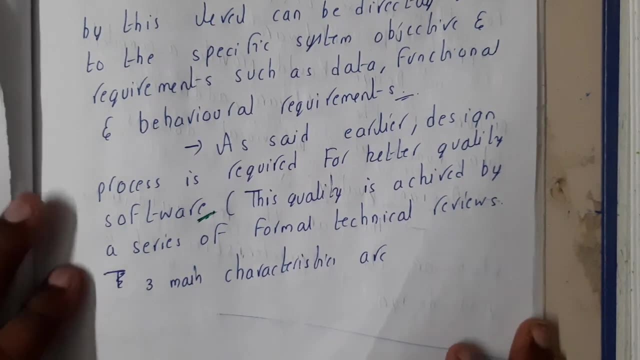 Similarly, as I said earlier, design processes required for better quality of software. So, basically, if you are planning to have a good quality of software like it should be user friendly, it should be easy to understand and everything You need to do the designing process in a perfect way. 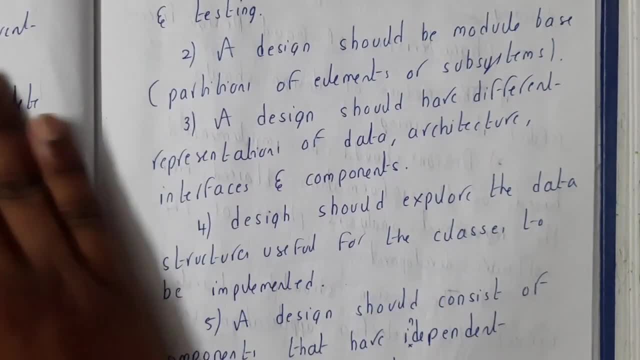 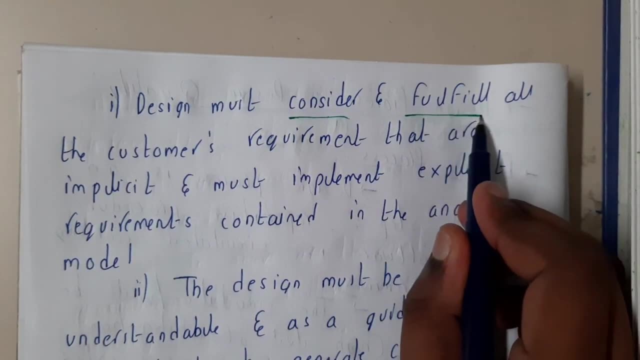 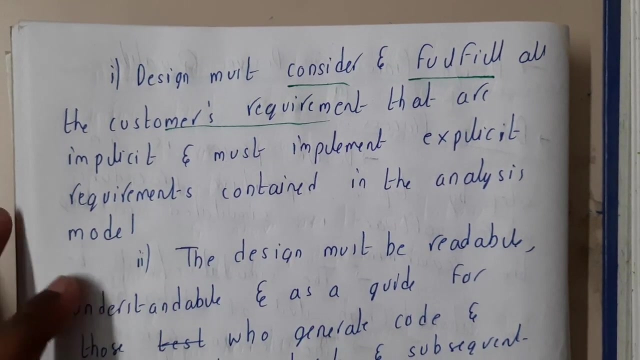 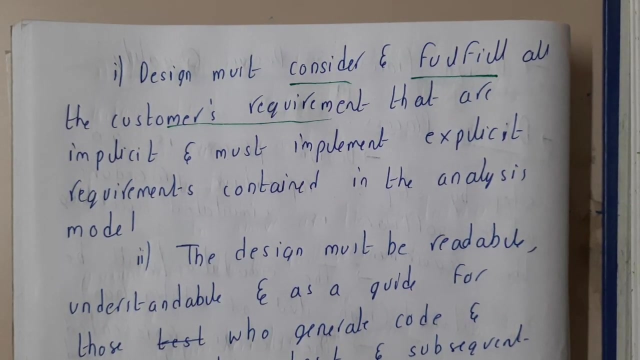 So there are totally three main steps, guys, okay, or three main characteristics, you can say so: design must be considered, consider and a full and fulfill all the customer requirements. So basically, once you are in a design stage, the next stage is coding, as if you start coding from this design. if the design is not appropriate, based on the user requirements, then the whole project will be a big flop. 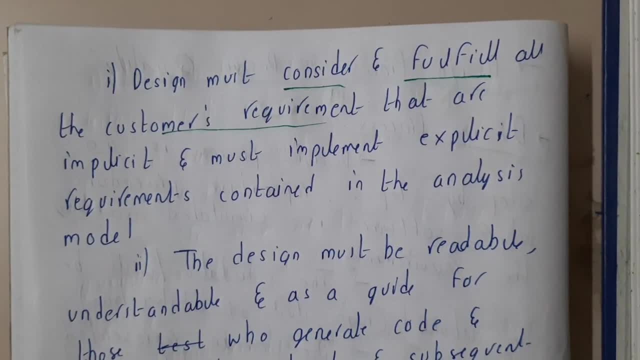 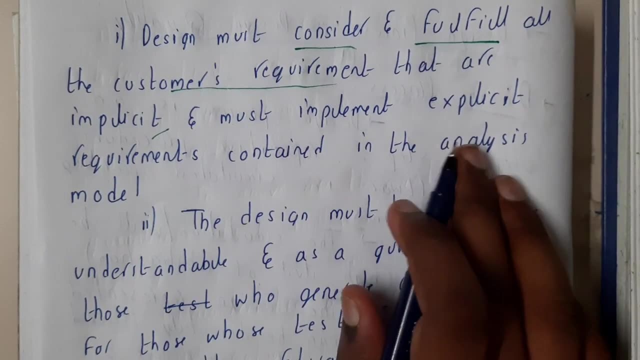 So that is the reason why we need to make it perfectly, So we need to fully. it should be exactly according to the customer requirements that are implicit and must be implemented: implemented explicit requirements contained in the analysis model. Okay, So it should have everything that the customer wants. 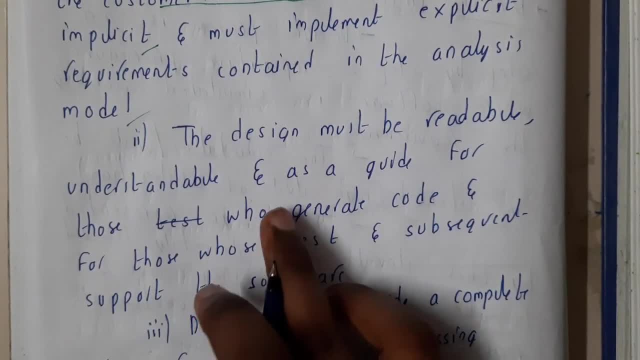 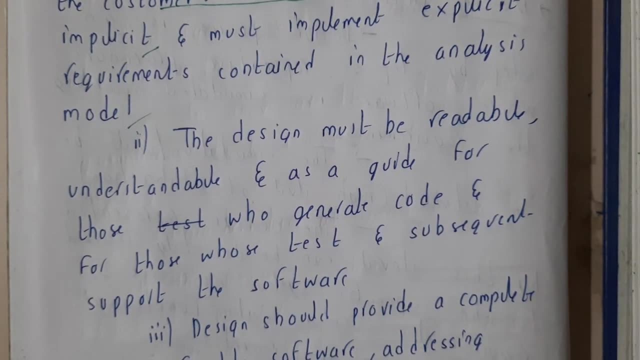 Okay, That design must be readable, understandable and as a guide for those who generate code. So basically, here we'll be saying creating something like a guide. Yeah, So we'll be doing it in this way. Then you do that.